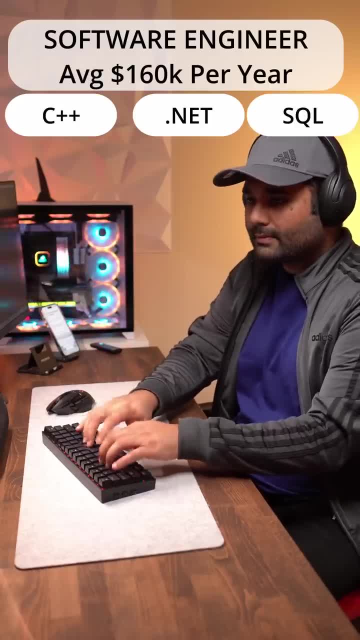 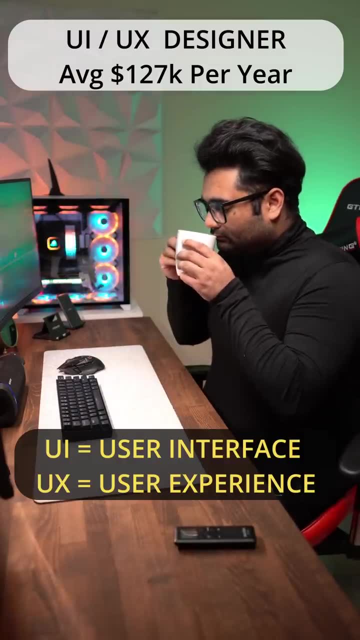 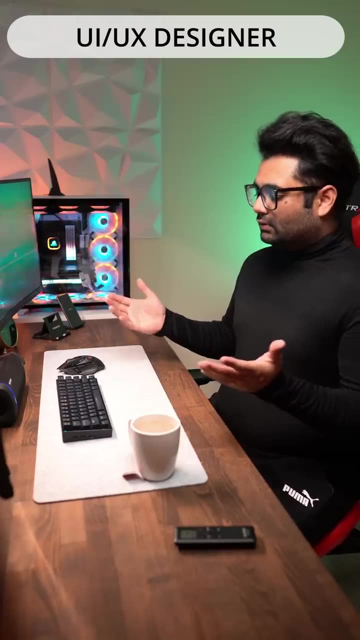 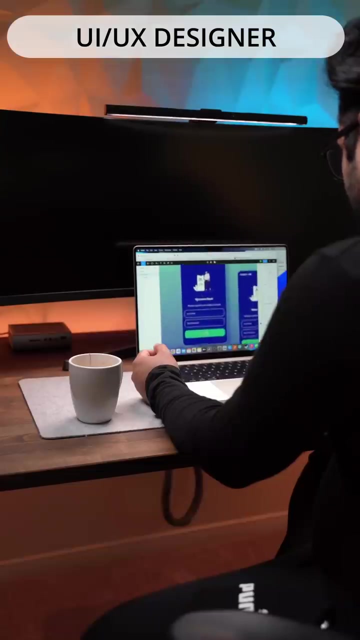 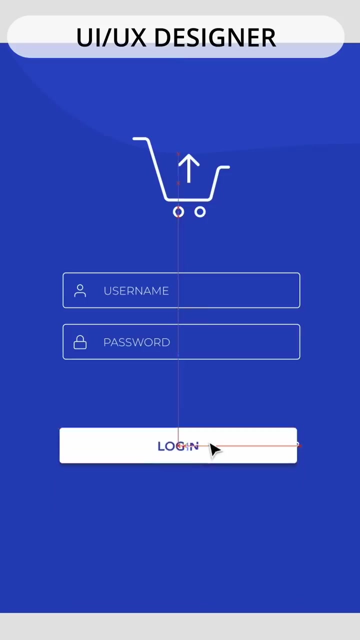 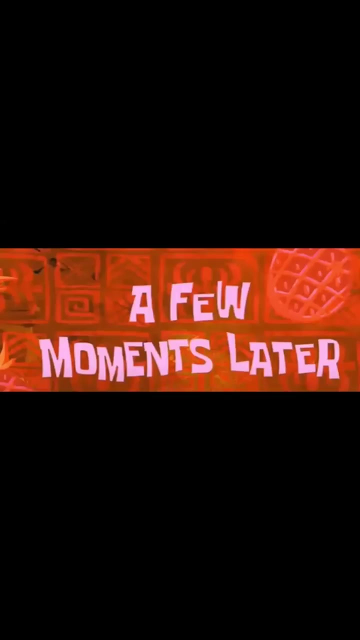 Oh my creativity juice. I can't work on Windows. I'm a designer, I need Mac. Hmm, I think I'll move it up here. Perfection A few moments later.